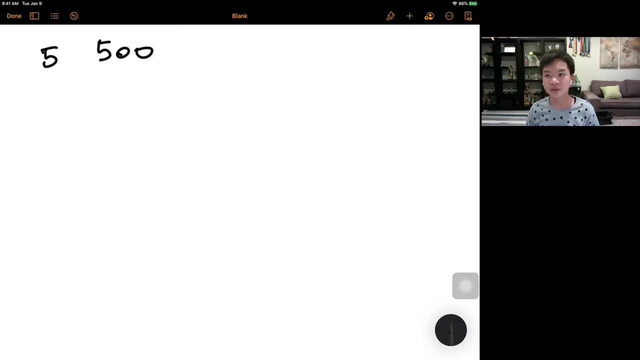 So one solution would suggest to be looping through each of the numbers from a to b. So we could loop through from a to b And then we could check if that specific number Is both a palindrome and a prime. So if it is, we can just print it out. 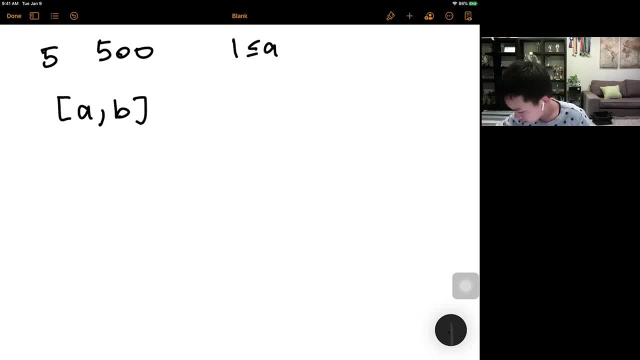 But then, since both a and b Is in the range of 10 to the 9th power, this wouldn't like work, since this would like take too long. So then notice that a palindrome Since a palindrome. 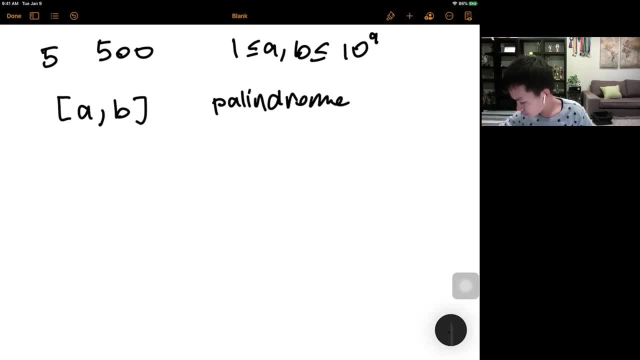 A palindrome Reads: Reads the same forwards, Forwards as backwards. Since it reads the same forwards as backwards, we can actually just generate the palindromes instead, Because instead of generating 10 to the 9th- like at most 10 to the 9th number of numbers, 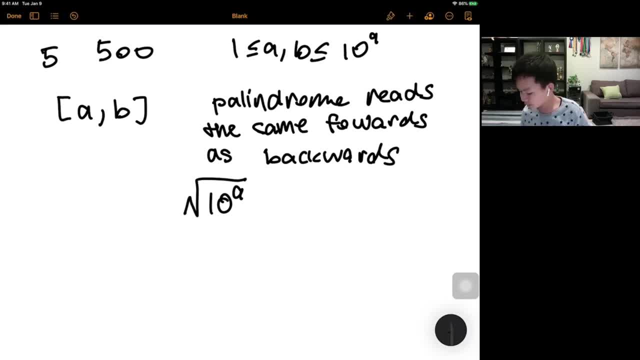 we can just generate the, basically the square root of this, Because, um, we're basically just generating the first, like, let's just say, if it's 10 to the 9th, we generate the first 5 digits. 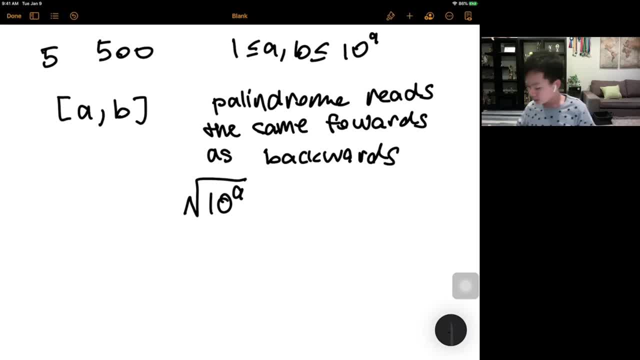 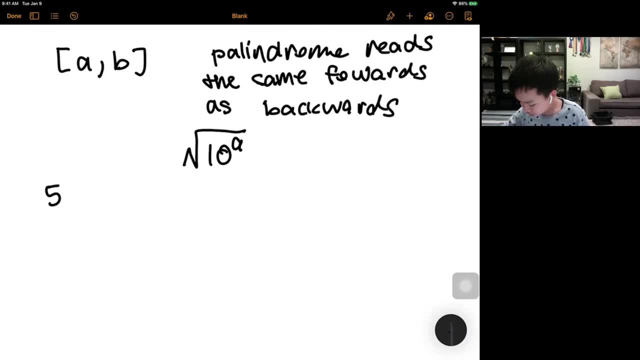 And then the rest. we know how to, since a palindrome reads the same forwards as backwards, And then we just check if this is prime. And what I mean is that, for example, if you want to generate a 5-digit number, 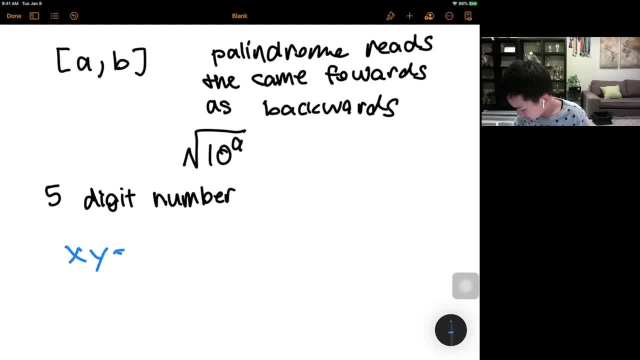 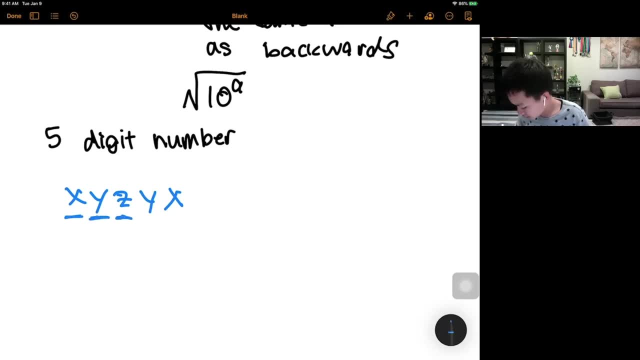 Notice that it has to be like x, y, z, y, Like x. So then we loop through all possible x, y and z. So then this can be from. This can be from 1 to 9.. 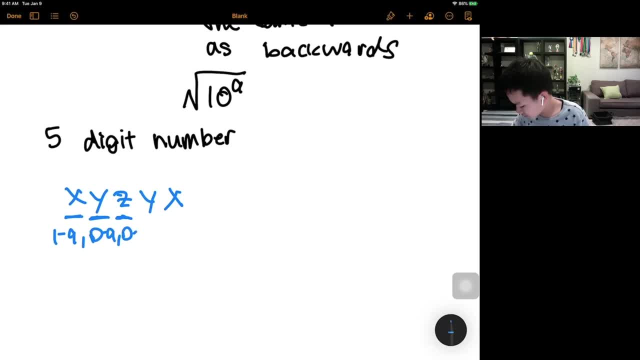 This can be from 0 to 9.. And this can be from 0 to 9.. And since this takes only like 10 to 3, like this would work And we only need to like generate half the digits. 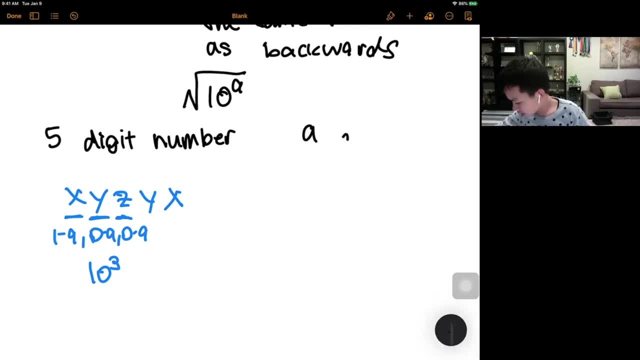 Another example is: let's just say we're generating a 9-digit number, A 9-digit number, Okay, so it has to be x. Or actually let's use a, So it has to be a, b, c, d, e, d, c, p, a. 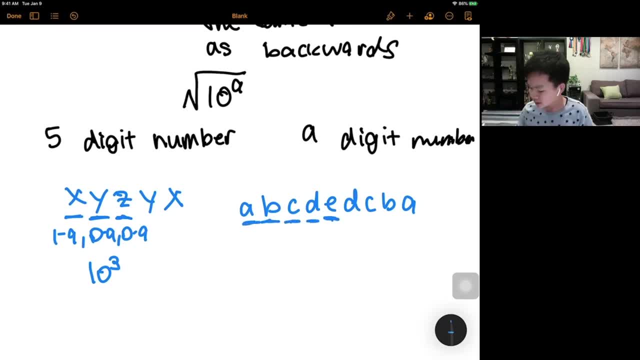 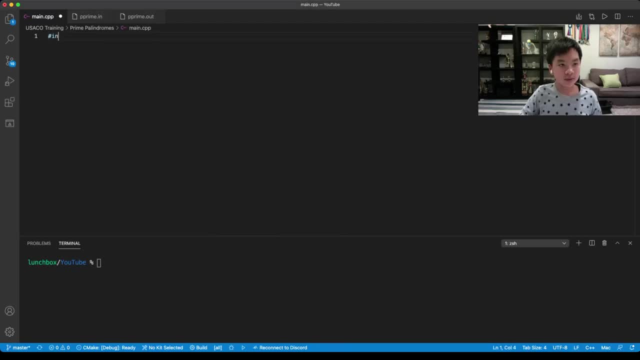 And we only have to generate these numbers. Okay, so that's basically it, And here we go. Okay, so let's include. Okay, So we have our a and b, So we're reading from P'. Okay, so we need to read a and b. 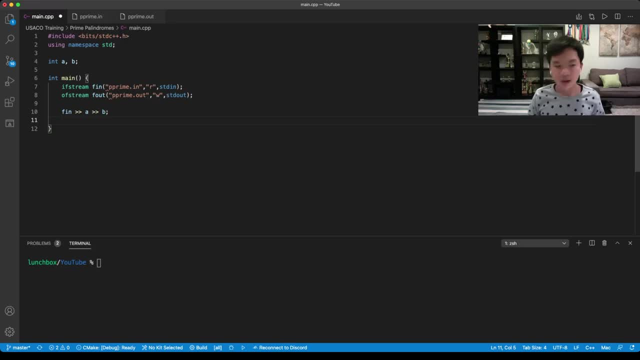 Okay, so now we need to generate our numbers So we can actually write them out separately. Okay, so we can. basically We can have a function. We can actually just write it out here. So here we need to first do our 1-digit numbers. 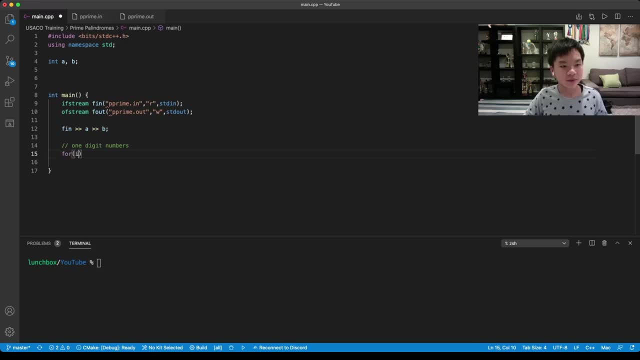 And this we can do. So we only have one variable. So if for i and- And I'm actually just going to use macros, Since it'll make this faster- A x, Okay, Okay, Okay, so now I just need to do. 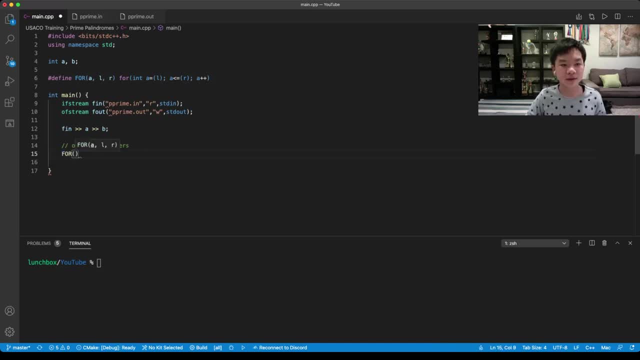 So okay. So for 1-digit numbers it can be from 1 to 9.. So for i: 1,, 9.. Okay, so basically you know that your prime or your number is i. Okay. so, basically, if you, 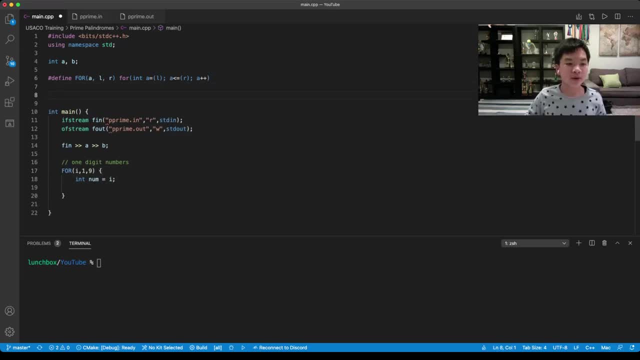 So we need to make a check function to make sure, like this, is a Both the prime and it is also in the range of a to b, So we can go check. Let's call this check, So we're given a number. 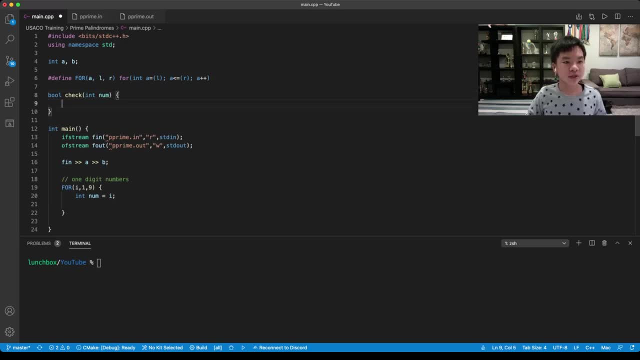 Okay, Okay. so first it has to be in the range of a, In between a and b. So basically, if number is less than a or the number is larger than b, then you can return false. So now we need to check if it's a prime. 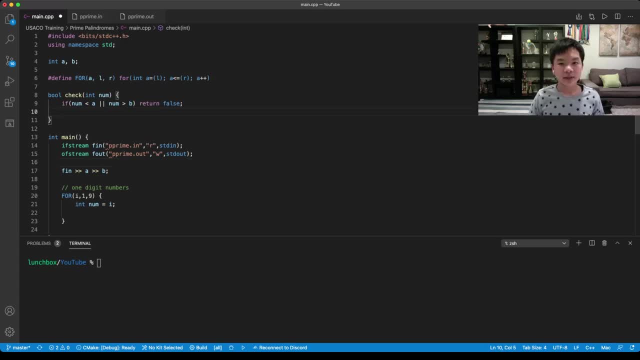 Okay, so to do that, we can actually check it in log n, I mean square root of n. So we can do this. Okay, so it'll be 4.. We can do 4i. 1. Let's call. 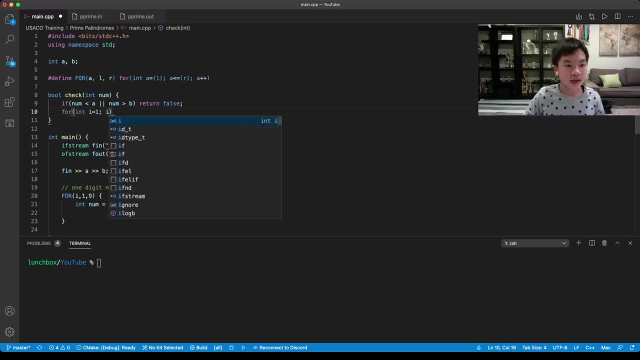 Or we can actually just make a So for i equals 1, i times i has to be, Or i has to be i times i has to be less than or equal to num. Okay, so if num mod or if it. 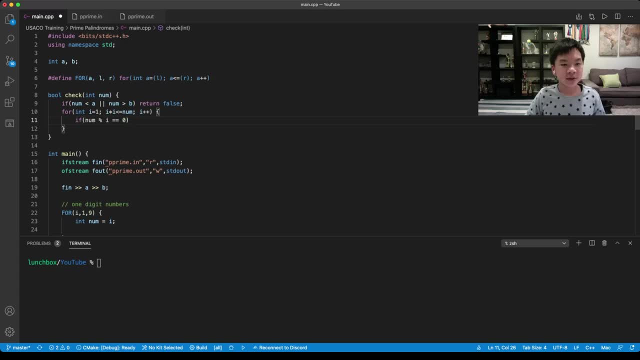 If a mod i is equal to 0,, then it means that it has a divisor. then you can return true, True, Else. then you can return false, Whoops return Okay. So now, basically. So, basically, if check, 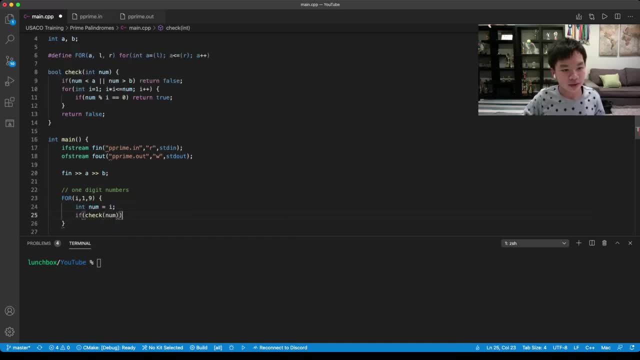 check num, then you can basically append this to your answer. So let's call this a vector of integers And you can answer the push back. i And notice that Basically, Since the last digit of a prime, or basically we can phrase it like this: 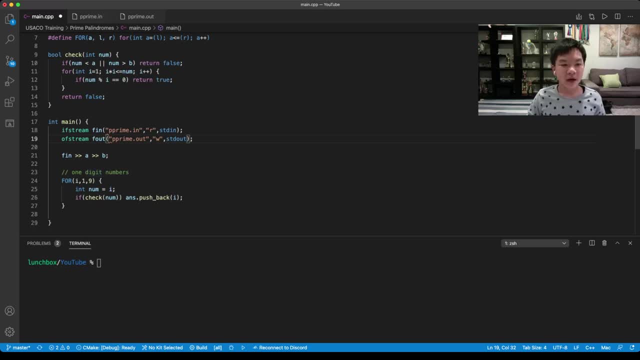 A prime like number always has to end in a Like, in a odd number, except for 2.. So we can actually Just use that to like, speed up the cases, So we can also make another one. So basically let's call this PRI. 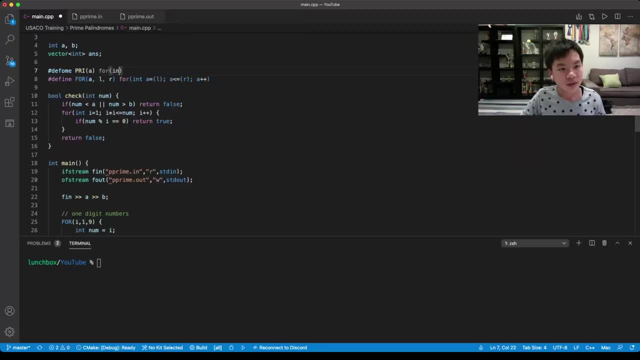 So we can call this a. So It'll be a equals 1.. a has to be less than or equal to 9.. And then you would just increment this by 2. Or this is- Let's actually call this- odd. 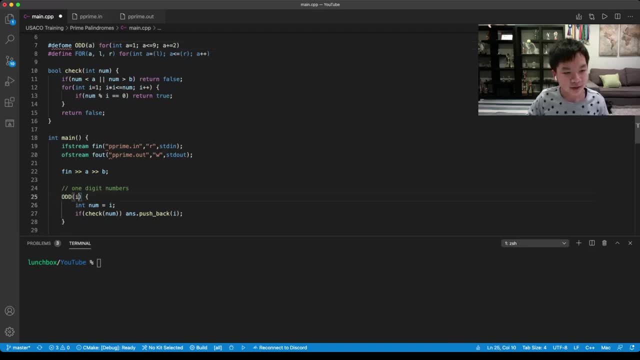 So now over here we can just do odd of i, So we basically only generate the odd like integers of i. Let's see, Okay, let's define, Whoops, Okay. So now we need our 2-digit number. 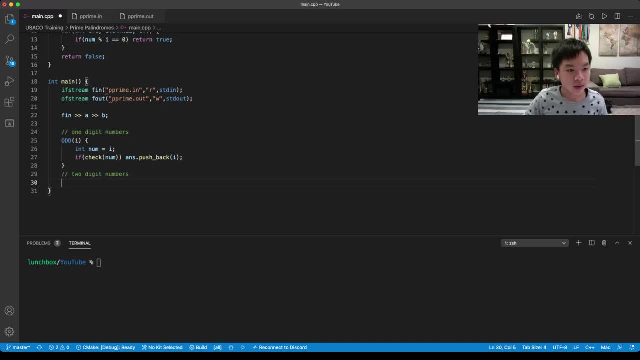 Okay, so basically we have Basically odd, So our first digit is i, So we have our number equal to i times 10 plus i And then. so basically we need to If checkNum, then we can push it back as well. 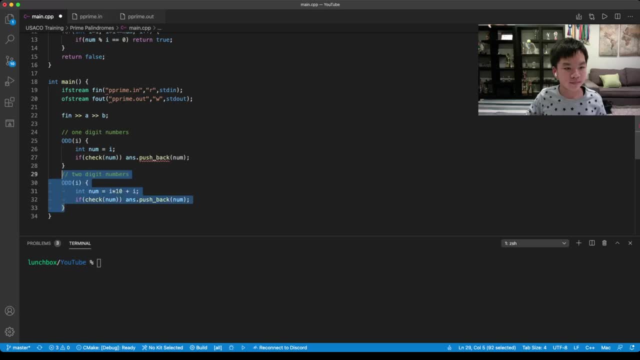 Yeah, this should actually be NUM. Okay, so now we need our 3-digit numbers. Okay, so this is our first digit, So it would be i times 100.. So now we also need our j times 10.. So we can. 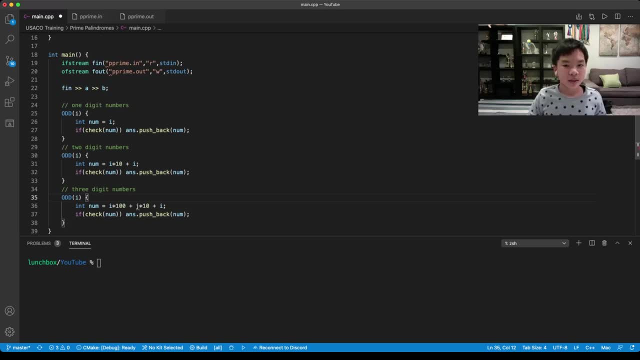 And j can be in the range from. It can be in the range from 0 to 9.. So we can do 4j09.. Okay, so that is our 3-digit numbers. 4-digit numbers: Okay, So the 4 would be the same as the 3-digit numbers. 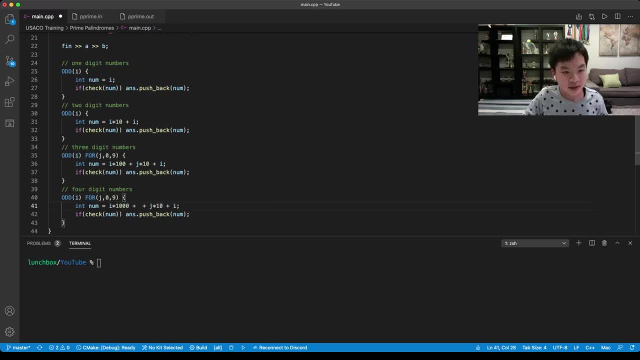 but then this would be 1,000 plus j times 100.. Okay, so now we need our 5-digit. Okay, so we have our odd, And then we also need our k Whoops, k09.. And here we go. 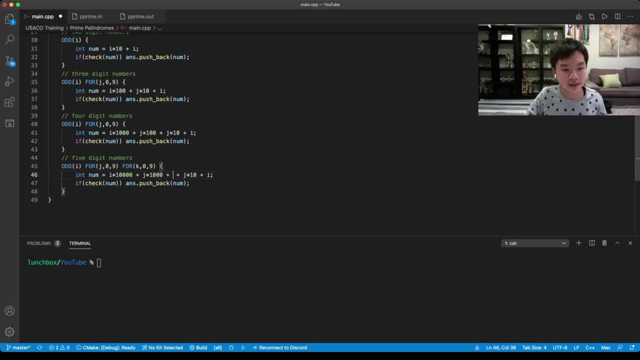 Whoops, this should say the same, And we need to add our k. Okay, so it would be k times 100.. Okay, so we have our 6-digit. Okay, so this would be The form would be similar. 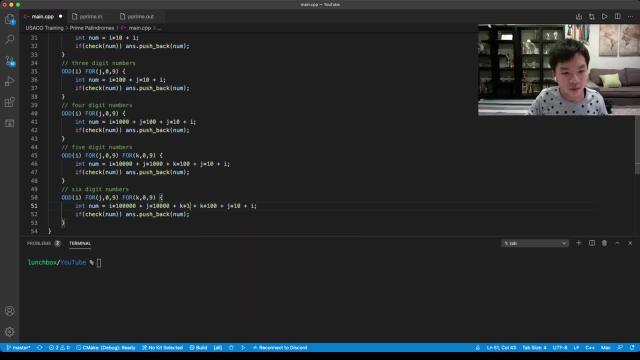 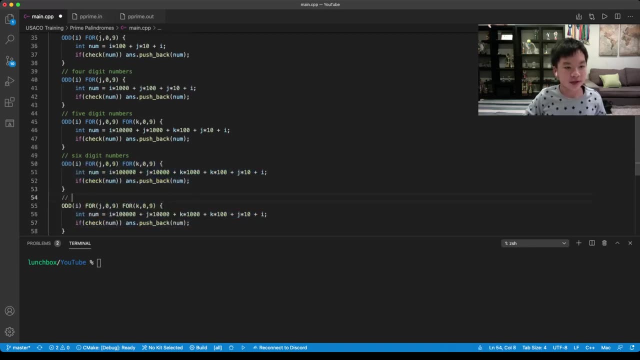 But here we would also add k times 1,000.. Okay, So we have our 7-digit numbers. So this should be. We should have, Let's call this l 0, 9.. We can do this as well. 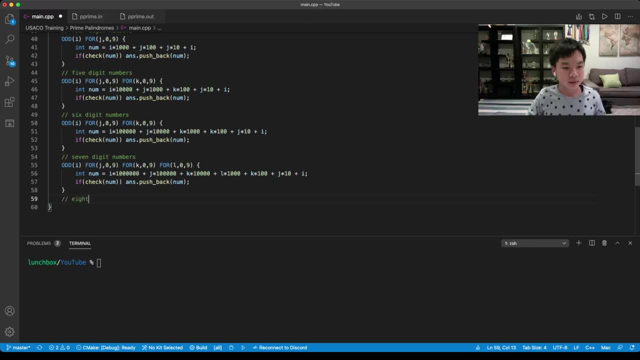 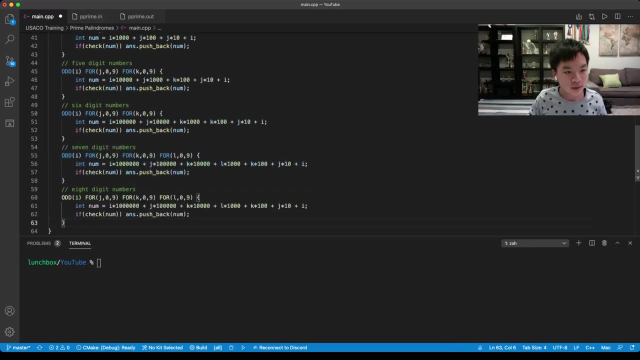 Okay, now we have our 8-digit numbers. Okay, so our 8-digit number would be similar to our 7-digit numbers. The only difference Was that it would be Having one more l. Okay, for our last one, we have our 9-digit numbers. 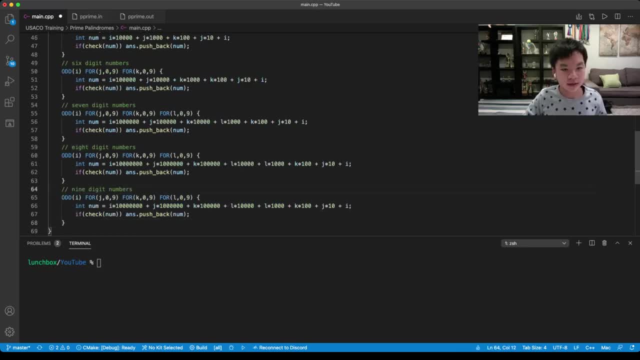 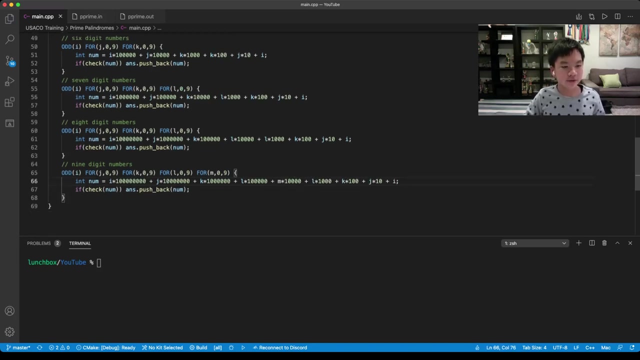 Okay, so 9.. And then Let's call this m, Then we would add another 1 as well, M times 1.. 1, 2,, 3, 4.. Okay, So now, after this, we just need to. basically, we need to sort our answer. 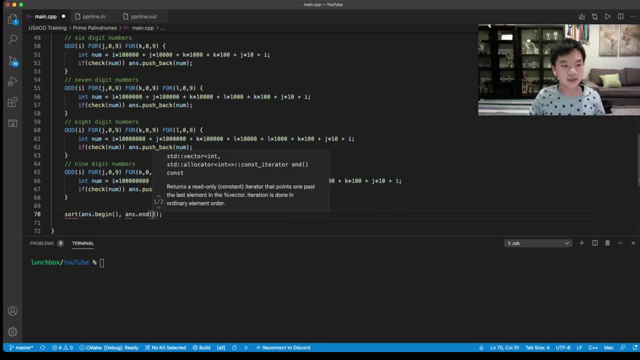 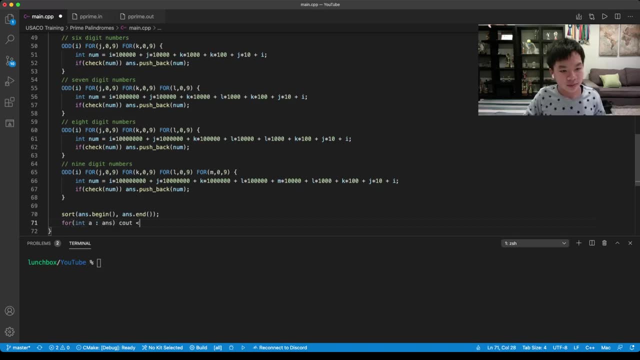 Whoops, m? m. My answer: m, m, m, m And so begin And n. Okay, So then we just need to print out our answers. So basically, for each answer we need to just First f out: 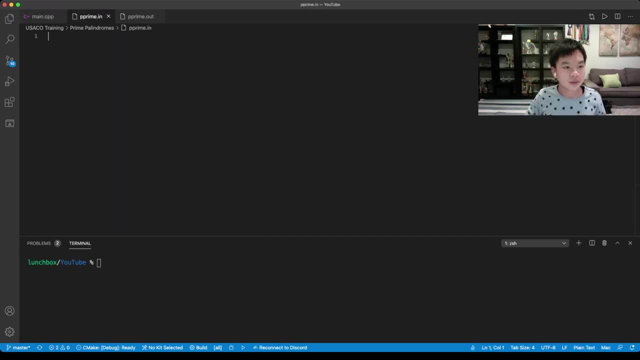 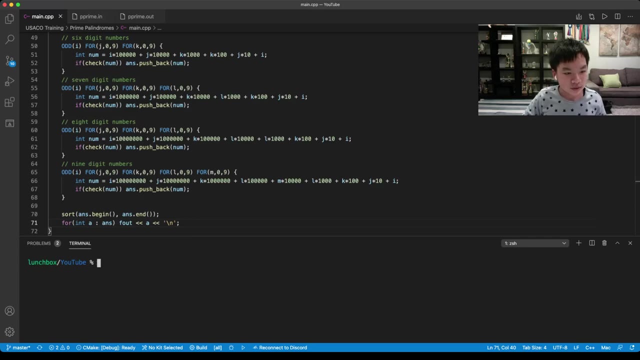 So f out A nblank. Okay, so let's get our input for the sample. we have five and five hundred, so so we have. this is the OCCO training and this is prime palindromes. okay, so let me just run this. 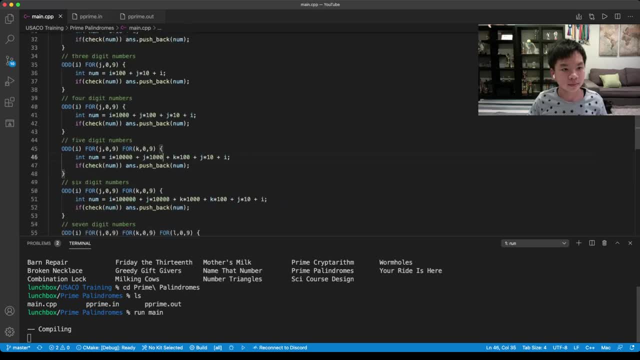 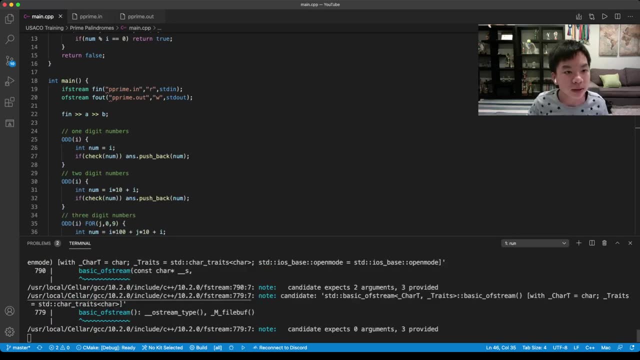 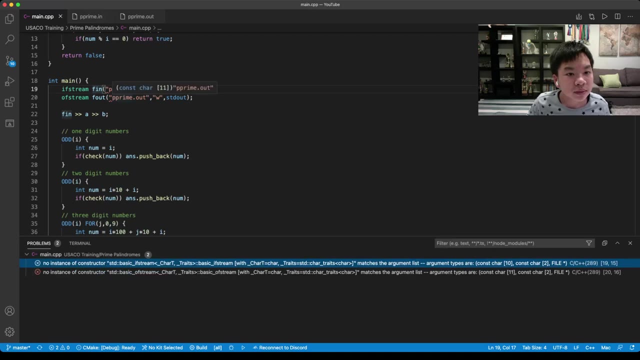 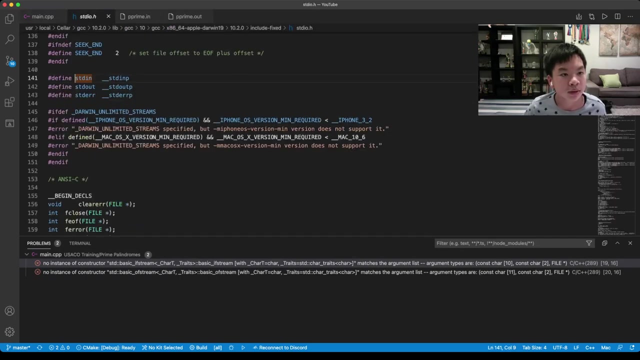 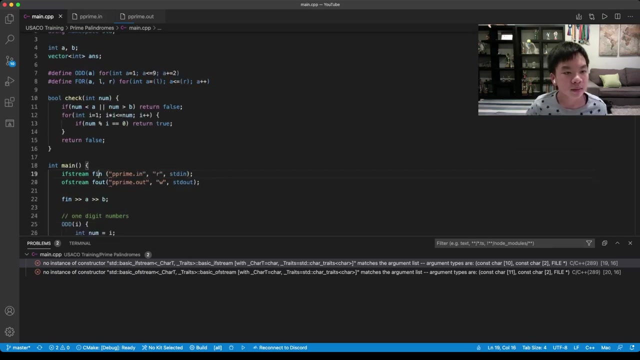 so there's an error. I'll let's see what it says: extreme. you prime that in okay, so the argument types are constant: char yeah, STD, yeah. so looks like maybe we can look at this extreme thing. oh whoops, looks like I did the extreme thing incorrectly. we actually don't need. 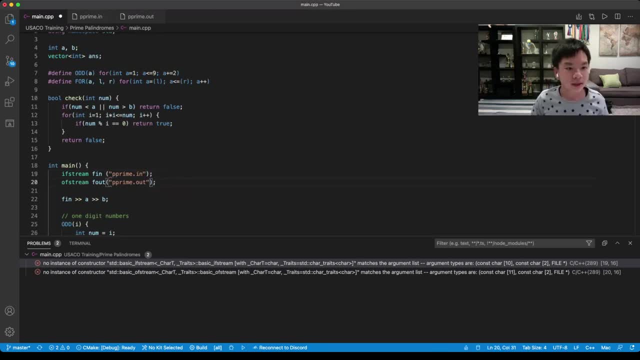 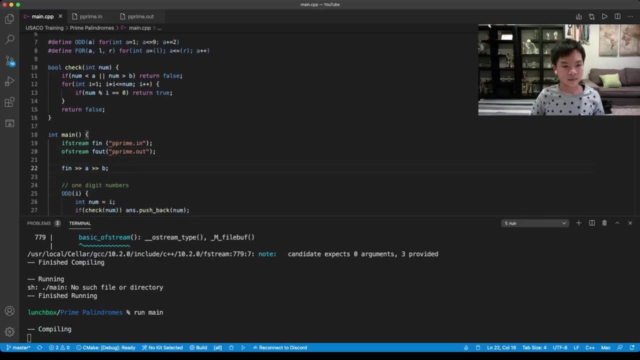 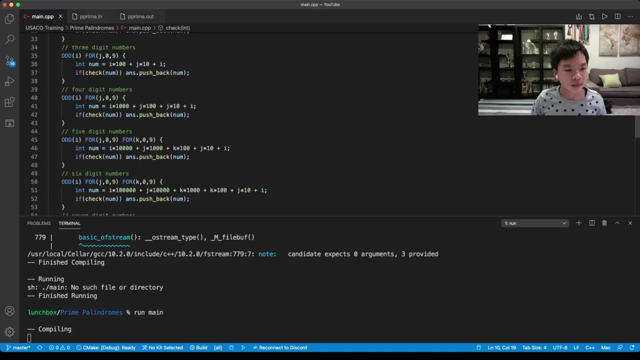 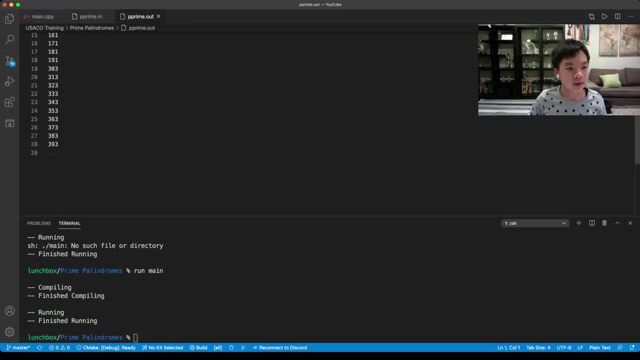 this: yeah, okay, let me run this again. you, you see it's compiling. okay, finish running over here. we see that these are all correct. wait, actually, three, nine, three, um, three, three, nine three isn't a prime, so let's, because it's a. uh, it's a. 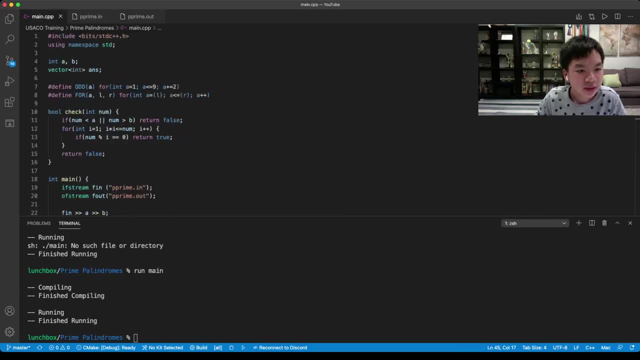 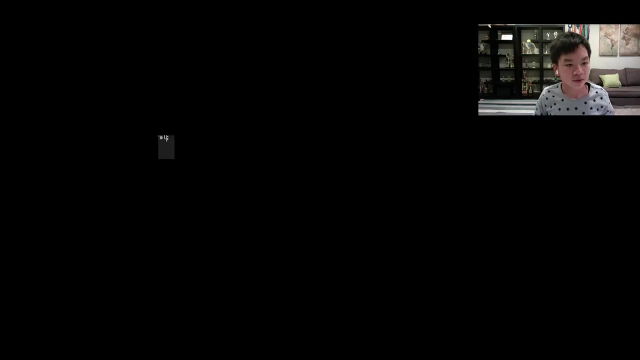 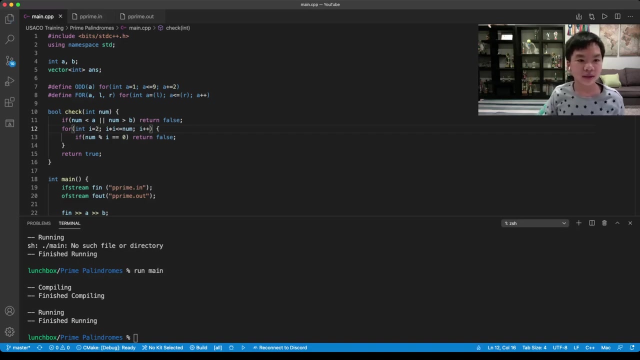 uh, it's divisible by three, okay, so if not three, oh yeah. so we actually did this, the opposite we actually have to do. um, you turn false and over here one, should it be included, since you know one? um, since, if you have one, since every number is divisible by one, so if it, 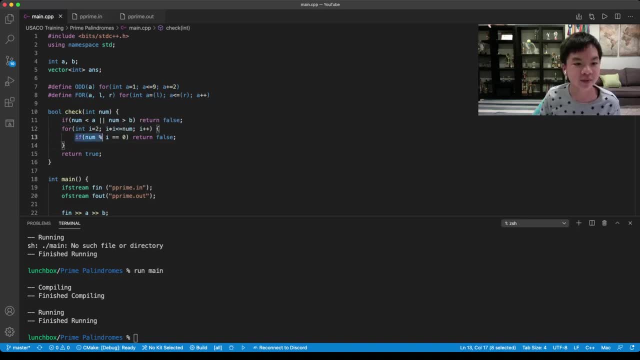 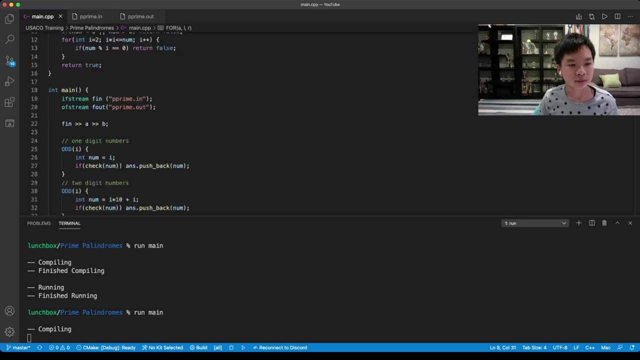 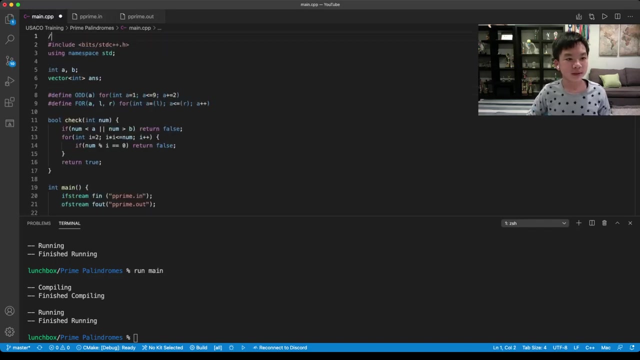 is divisible by one. so basically, this means that if it is divisible by a number, then you have to return false, okay? so let's run this again. okay, let's check this. okay, so it looks like that is right. I'm just going to submit it, okay, so 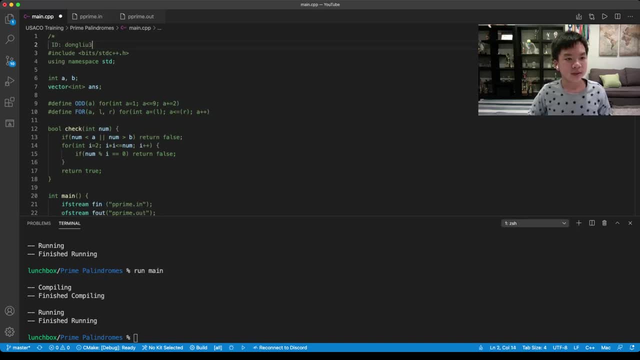 here's my id. this problem is people. I'm just going to submit it, okay. so here's my id. this problem is people. I'm just going to submit it, okay. so let's go back and see that I got that. okay, it's prime. this problem is people. 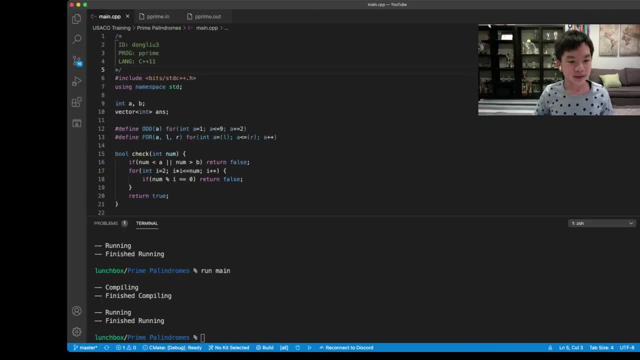 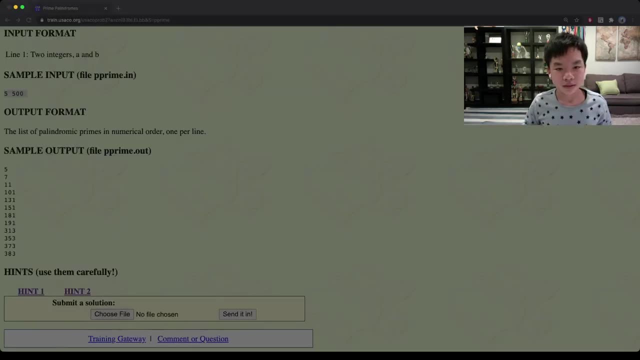 and I'm going to run this over anyway. okay, so this one is prime- yes, it's prime- and um, my language is c++ alone. okay, so here we go. okay, maybe a site code training. this is um prime power drums. okay, here we go. okay, so it looks like that is right. 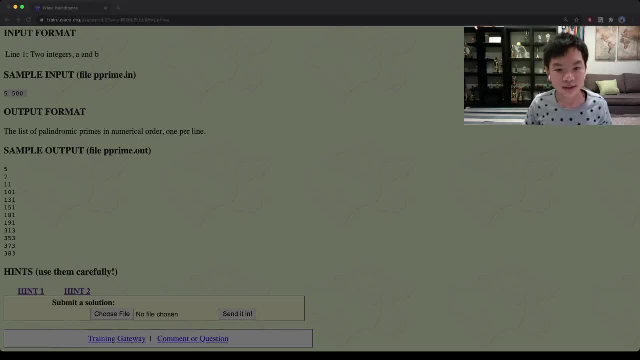 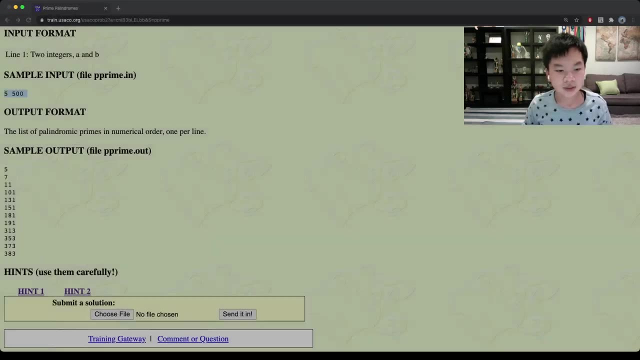 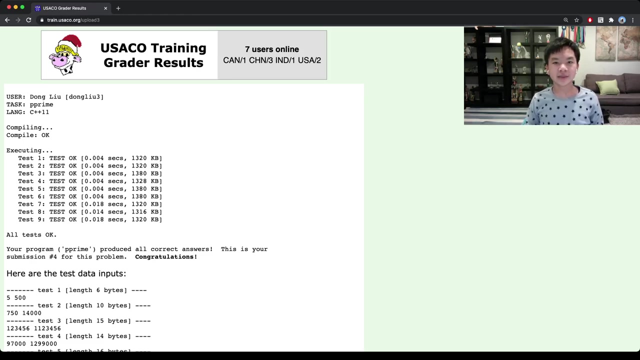 this has to be true in png. in png, okay. yeah, so it looks like that is right. okay, so here we go. I'm gonna type in, you know, this above: this is okay. this is prohibited. okay, so it looks like that is So. if you have any questions, feel free to leave them in the comment section below.